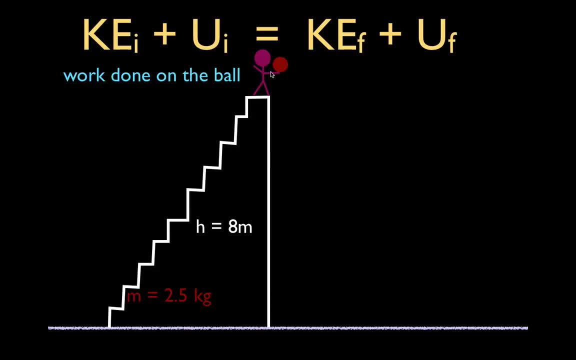 How much work do they do when they carry the ball from here up to here? Okay, now for work. we're going to start out talking about work. Work is the force times the distance times the cosine of theta. So we want to figure out what is the force, what is the distance and what is the cosine of theta. 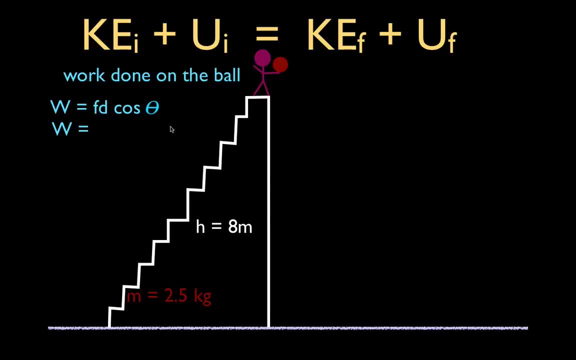 And then we can solve for the amount of work, The force. when you carry something up the stairs, when you carry something up a ramp, when you carry something up like that, you apply a force. That force is applied vertically and we'll call that the applied force. 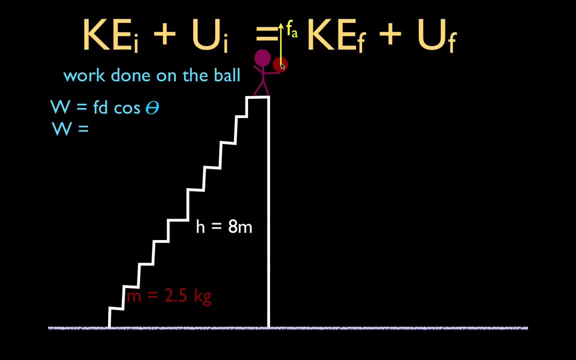 The force you apply is not parallel to the stairs, it's a vertical force. you're working against gravity. That is the applied force. That is the force that we're going to be talking about, But we don't want to put FA in there, because we can say that we know that that force that we apply, 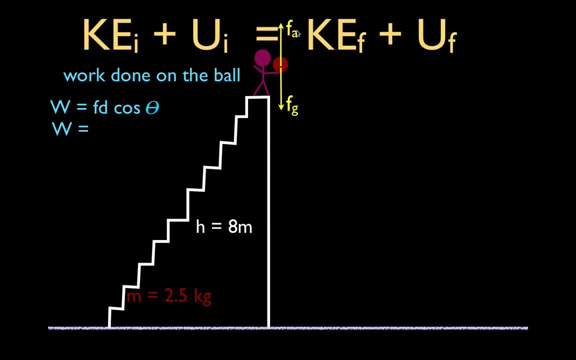 is equal to the weight of the force due to gravity on the ball. Okay, so the force that you apply is equal to the weight of the object in newtons, and we know the weight of the object is the mass times the acceleration due to gravity. 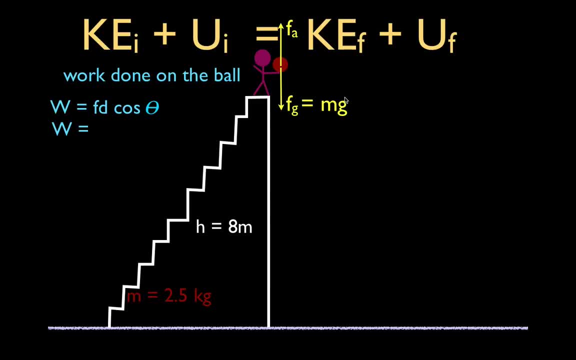 We have the mass. We know the acceleration due to gravity is 9.8 meters per second squared, so we can substitute in for the force. The force that you apply is equal to the mass of the object times the acceleration due to gravity. 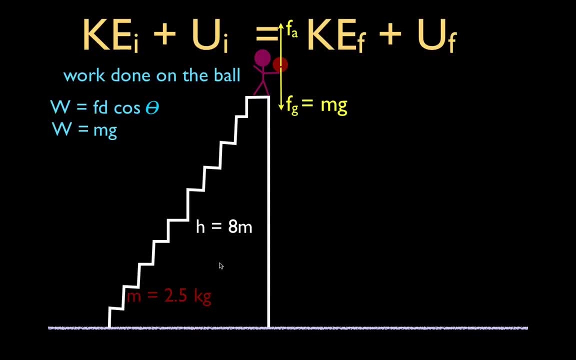 or the weight of the object. Now, what about the distance? Over what distance did we apply that force? Well, that force was applied over the height of the stairs. not the length, but the height. That's the change in y, the height, the change in the height of the object. 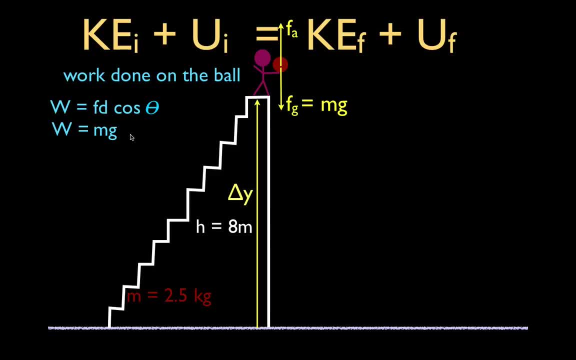 and we said that is 8 meters, so we can put in here m, g, delta, y. Okay, now the cosine of theta. What is theta? Well, the theta is the angle between the displacement vector and the force that you apply. 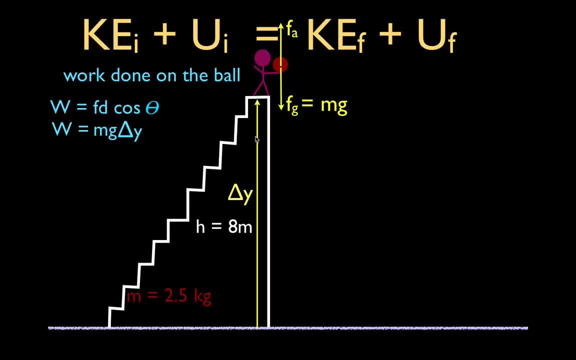 Not f, g, but the force that you apply. And these two, this vector and this vector, are parallel to each other. They're pointing in the same direction. so theta is 0 degrees, The cosine of 0 degrees is 1, so we could write m g, delta y, 1,. 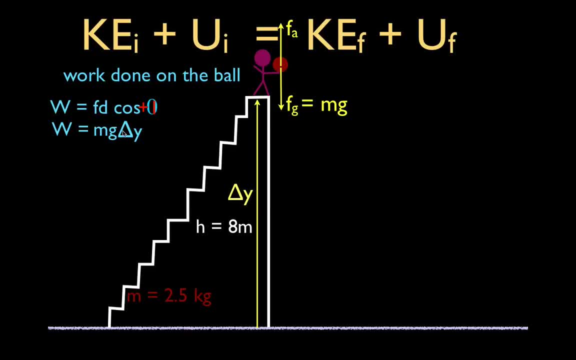 or times 1, we don't write that down, so we just have m, g, delta, y. Now that is the work. The work that you do on the ball is equal to the mass of the ball, times, the acceleration due to gravity times, the change in height. 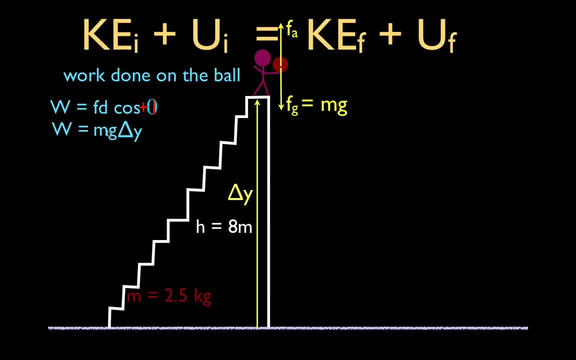 Now you may notice this equation looks a lot like the equation for potential energy, because when you have an external force and it's raising an object up, the amount of work you do is equal to the change in potential energy. and we want to keep that in mind because we were asked how much work you do on the ball. 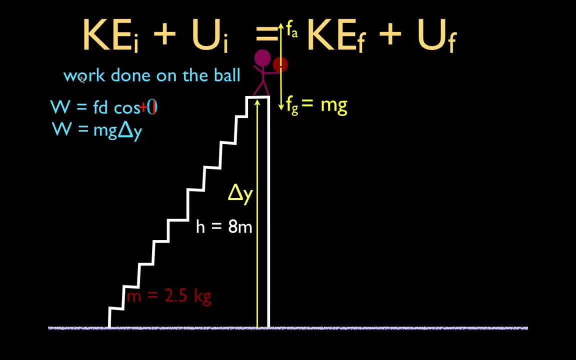 We could have also asked you what is the change in the potential energy of the ball? Okay, But we said this is in terms of work and mechanical energy, So we can now plug our values in the mass of the ball: 2.5 kilograms. 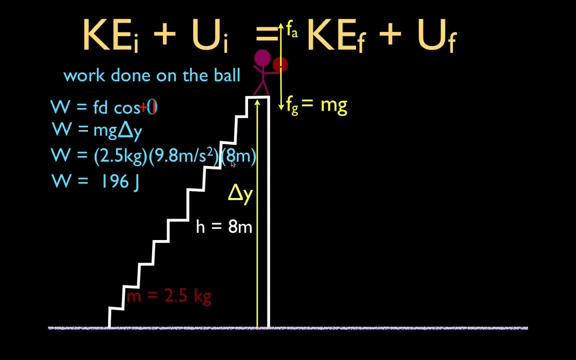 the acceleration due to gravity and the change in height, and we get that the work that you do on the ball is equal to 196 joules. Well, what happened to all that work? Where did all that work go? Where did all that energy go that you expended carrying that ball up those stairs? 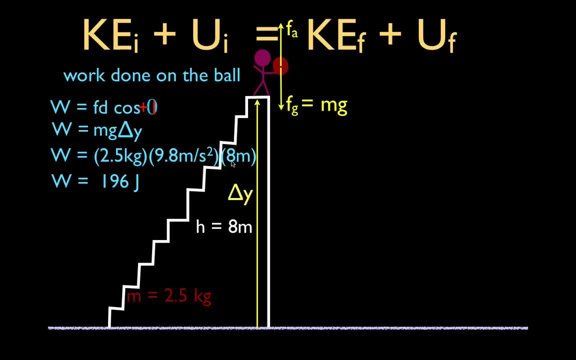 Well, that went into the potential energy of the ball and that means you gave the ball potential energy. And that means now, when we turn to our equation for conservation of mechanical energy at its initial position, we're calling this its initial location because we're going to drop it down. 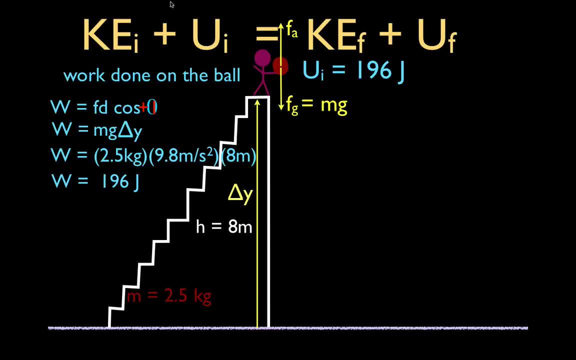 At its initial location, it has 196 joules of potential energy. Well, we want to use this equation. So what about its kinetic energy? Well, you're just holding it right there, It's not moving, It has no velocity and therefore it has no kinetic energy in its initial position. 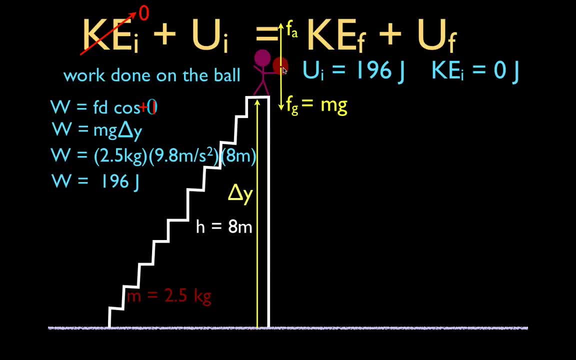 So we say that initial kinetic energy of the object is zero. That means its initial total mechanical energy or its initial mechanical energy is 196 joules. Now we're going to drop the ball down. It's going to go like that and it's going to go almost to the very bottom. 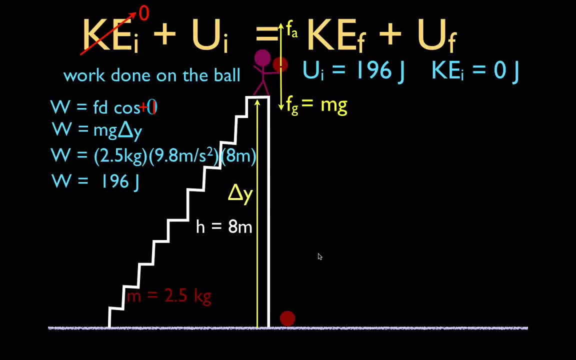 It's not quite touching the surface down here. We want to know what happened to the kinetic and the potential energy. So we want to know what is the final kinetic and the final potential energy. Well, when the ball fell down, the potential energy is due to the height, the position of the ball. 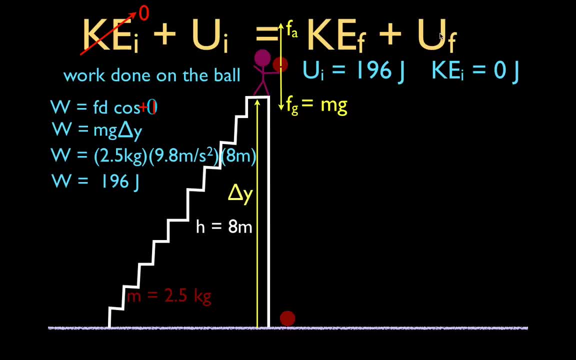 Now it has no height. It's due to the height above the ground surface. So now we know that its final potential energy is zero joules. Look, it had 196, and now it has zero joules of potential energy. Where did all that potential energy go? 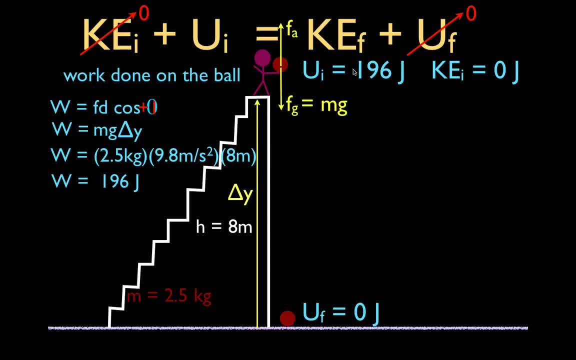 Well, as it fell, it gained velocity, It accelerated so that potential energy went into kinetic energy and it's basically lost all of its potential energy. So all of its potential energy was converted into kinetic energy and now it has 196 joules of kinetic energy. 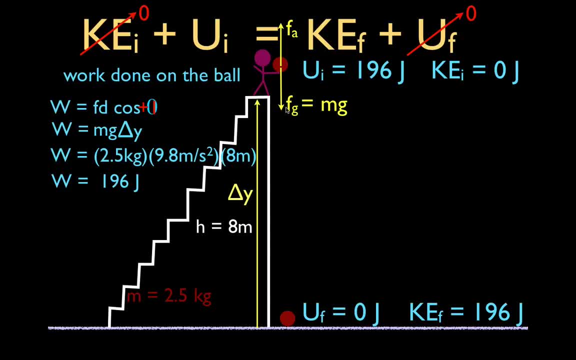 As it hits the ground, just before it hits the ground, as it fell through that eight meters. I realize here it's a little higher than eight meters, but we're assuming you bent over and you leaned right there and you dropped it from eight meters above the ground surface. 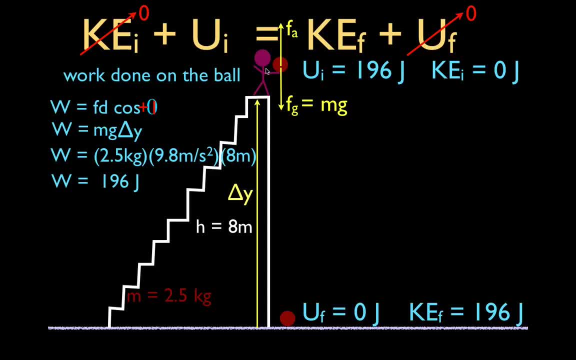 because that's officially the height of the stairs and that's how much you changed its height. So we figured out how much work. That was question number one Using our work equation: 196 joules. That went into the potential energy. 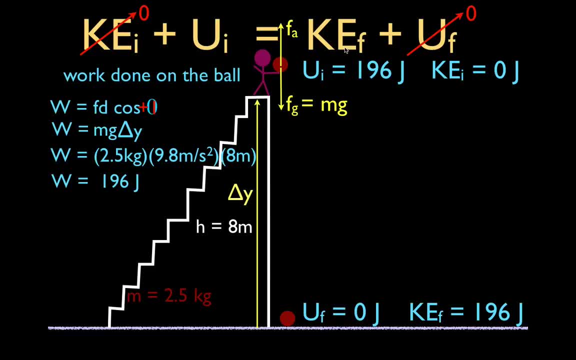 We had no kinetic energy. We used our conservation of energy equation and determined that it lost all of its potential energy and the potential energy was converted into kinetic energy- 196 joules, And you can see: if we add 196 and zero, that equals zero plus 196,. 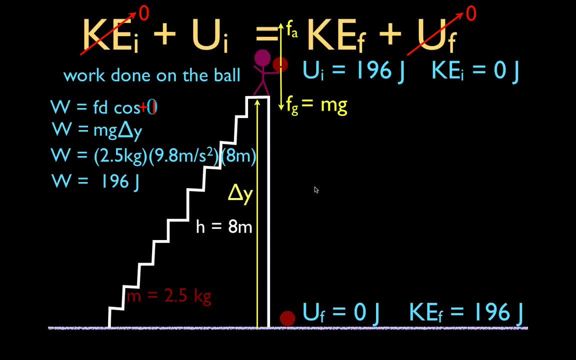 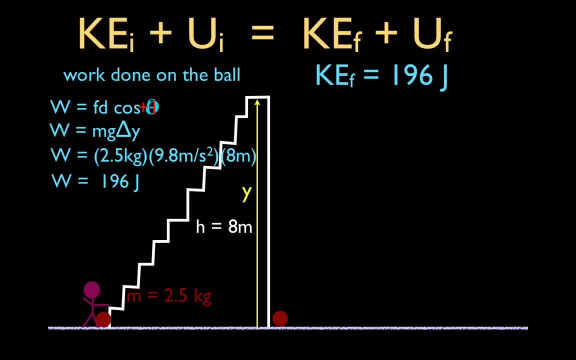 and we have conservation of mechanical energy, And that's basically true because we're saying there's no friction of ignoring air resistance. Now we can solve the third question and we can answer. the question is: what was the final velocity or what is the final velocity of the ball after it falls through that eight meters? 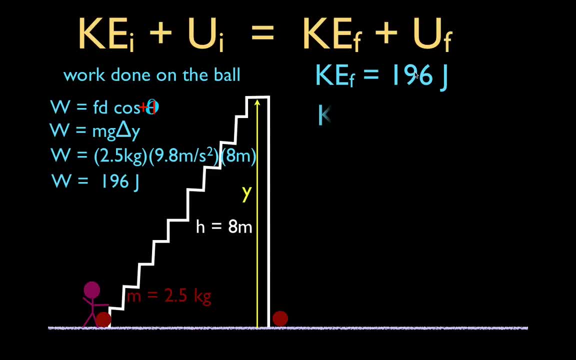 Okay, the kinetic energy we said is 196 joules. Well, we know the equation for kinetic energy is one-half mv squared. So now we can solve for this final velocity squared, or the final velocity actually, because we know the kinetic energy: 196.. 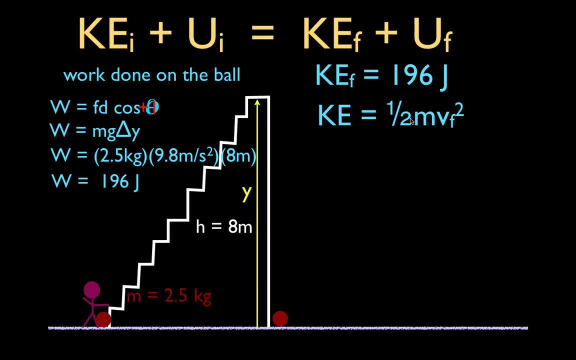 We know the mass and we can solve for final velocity using this equation. Okay, So we're going to use our kinetic energy equation and we're going to solve for the final velocity. To do that, we're going to multiply each side by two.